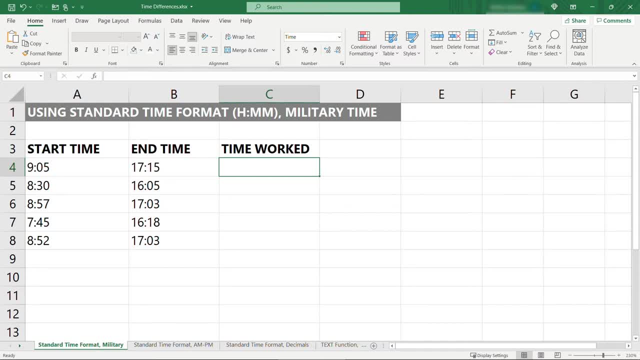 Hi friends, thanks for watching. There's all kinds of situations where you need to calculate the difference between times, and Excel makes it easy to do that. I've got five different examples for you here. Let's start with needing to calculate how long somebody worked, based on their start. 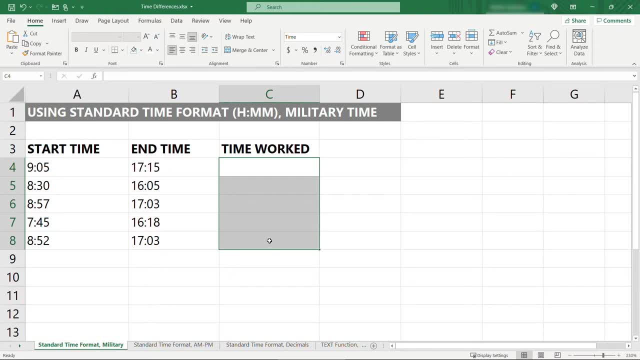 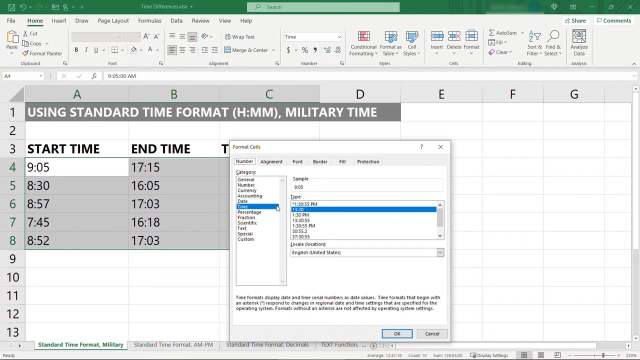 time and their end time. In this example, the first thing we're going to do is make sure that our cells are formatted correctly using the correct time format. So I'll just select all of those right-click format cells, and here we want to go with the time category and then over here. 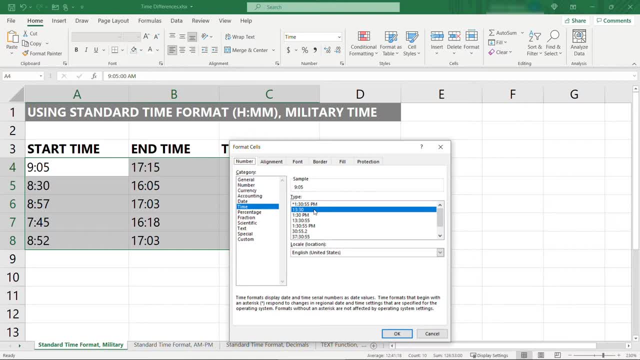 the 1330,, meaning it's using the 24-hour time format rather than 12.. Some people call it military time. In this case, we're not worried about the seconds, but there is a seconds option as well. if you have something more precise that you're trying to calculate, We'll go back to the 1330,. 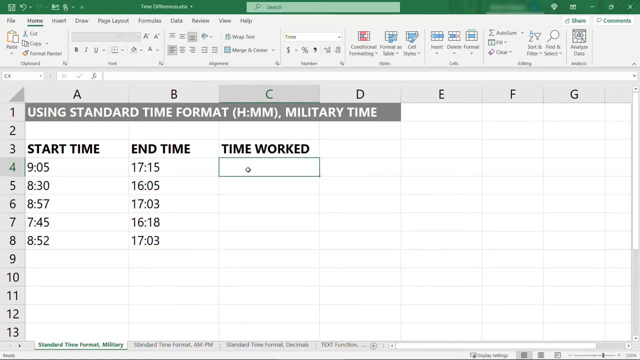 click OK, and then all we need to do now is a little bit of math. So hit the equals button. This is going to equal end time minus start time. Enter. And here time worked is eight hours 10 minutes. Now to copy that down to the other cells, you can either just: 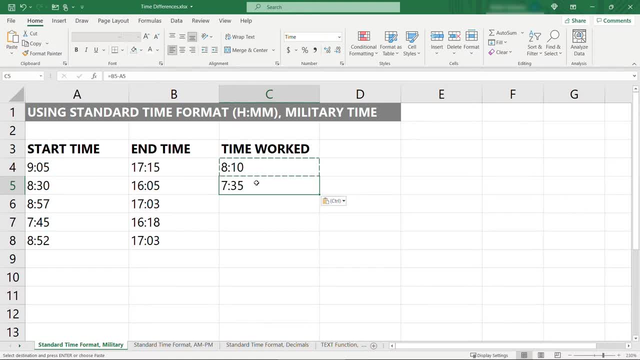 do a copy control C and then paste control V, or you can also pick this up on the lower right here, this little handle, and drag it down to the other cells. How easy was that? Just a simple subtraction. All right on to my next example Here, rather than using the military time or 24-hour time, 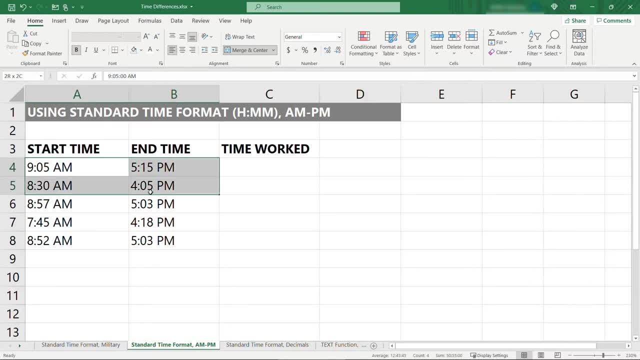 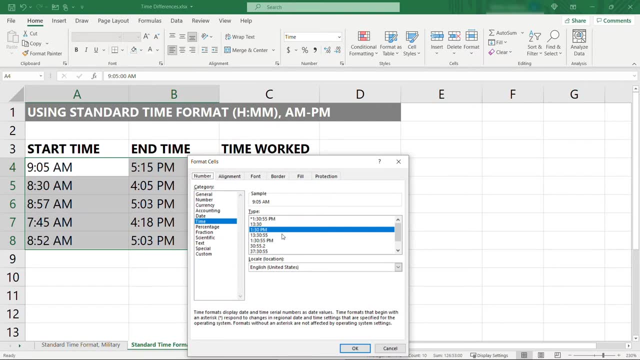 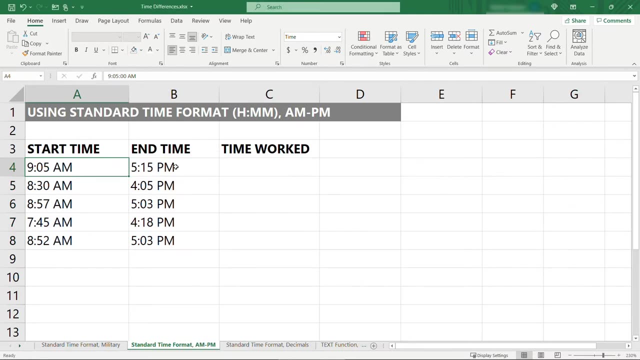 format we're using am and pm. If we look at these cells here and right-click format cells, you'll see the 130 pm here rather than the 1330.. And even if you typed in over here, for example, if you did 1700 military time. 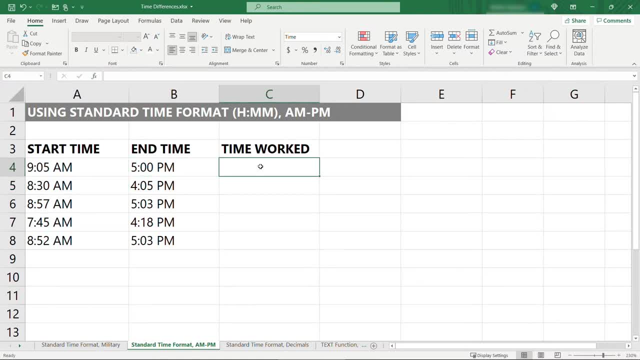 you'll see that it formats to the am pm Over here for time worked. this is actually still what we had on the previous tab. We don't really need an am pm here. That wouldn't really make sense. 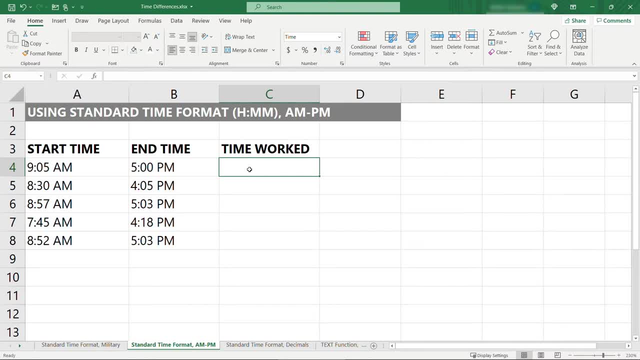 We just want the total hours and minutes that somebody worked. Okay, the formula will be exactly the same. So B minus A, So seven hours 55 minutes. The time is actually different than this last one. You might be thinking: why isn't it 810?? It's because I changed that end time. 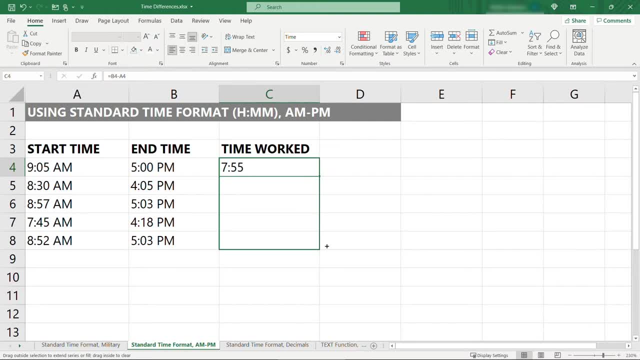 To be five o'clock sharp. The rest of these should be the same, though. if we drag the formula down And there we go. Okay, but what if you needed these to be in some kind of a decimal format where you're adding them up Rather than seven hours and 55 minutes? you need something like: 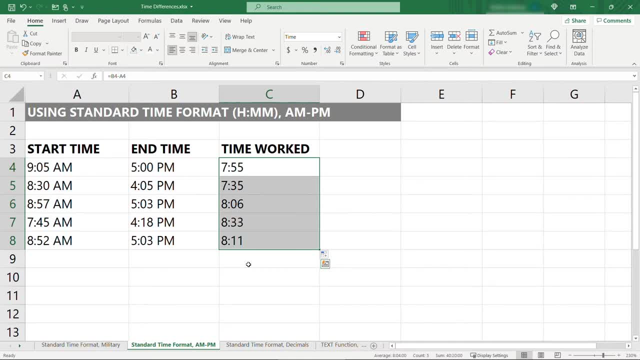 7.9,, let's say, as a decimal. Easy to do that as well. Let me come over to this other tab. This one will involve multiplication and a different format on your cells. Let's start with the formula. So this will be. 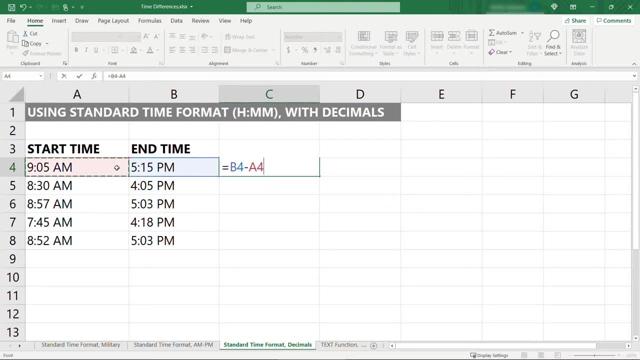 B minus A, And this time we need to multiply by 24 for hours, So times, or the asterisk 24.. If we drag this down, you'll see we get that there in the decimal format. But something else that you also need to double check is that you're using number here. 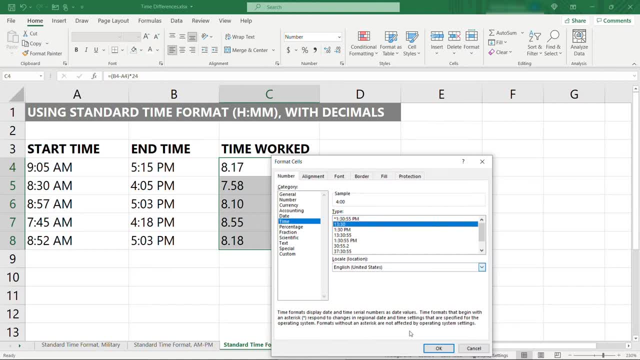 rather than the time. If you still have this in time, like we did before, it's going to give you something really odd. It's not going to look right at all. So here is the magic trick. was the format coming up to number? 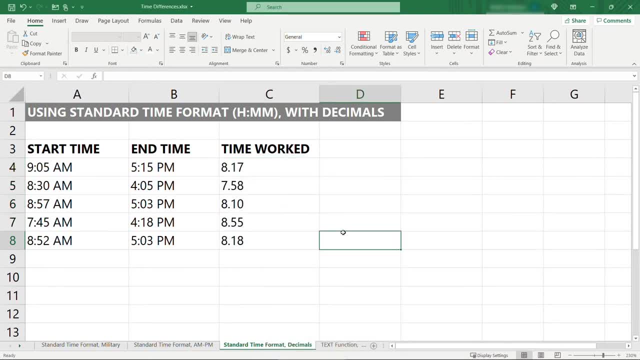 having two decimal places and click OK. Again the formula. there. you're multiplying it by 24 to get hours, and then you needed to change the format to be displayed in numbers rather than a time. All right, moving on to the next example, What if you needed just hours here? If we look, 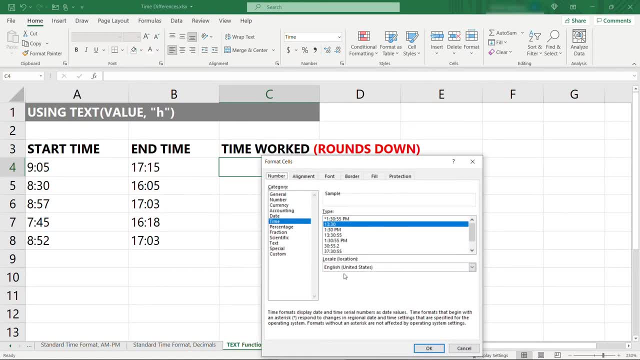 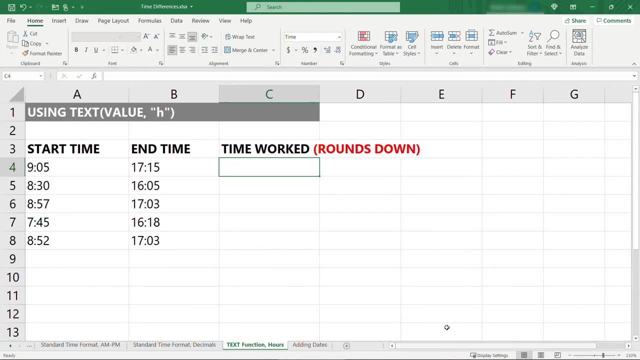 at our time format options, you'll see we really only have hours colon minutes. there's nothing just for hours here. So if you want to do that, you can use what's called the text function Here. just type in equals text. The value is going to be that same formula. we've 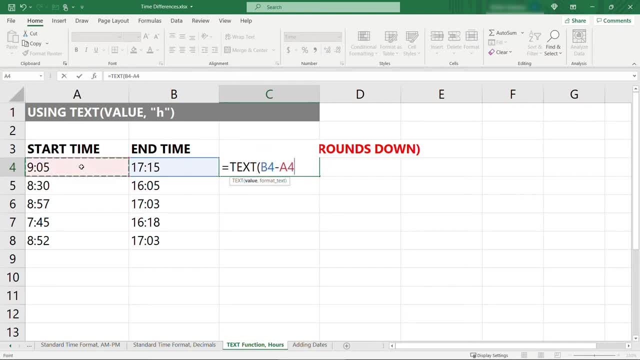 been working with. So B minus A comma, and then the format in quotes, put an H and then close this off with a parenthesis. And there you go, Dragging our formula down. you'll see, we have that in just hours now And a note as called out.